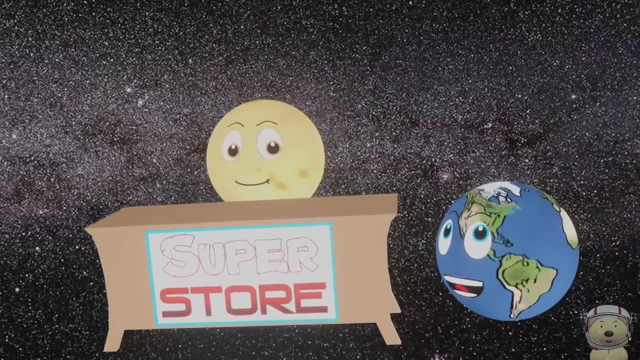 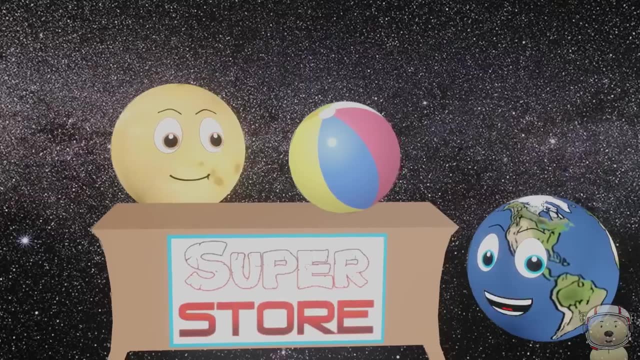 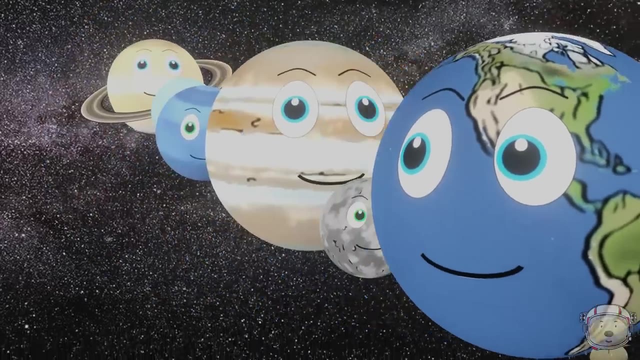 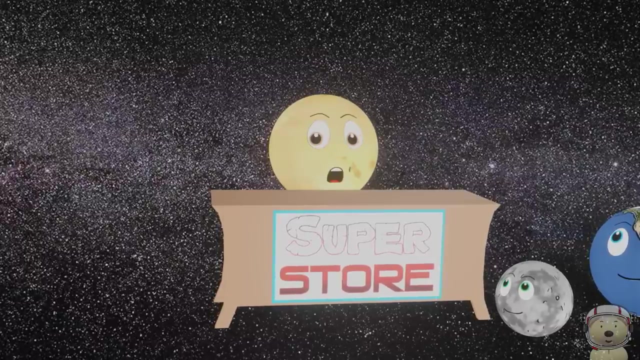 Try me. Well, I'm the only planet with liquid water in the entire solar system. I wanted a beach boat. Uh, Uh, How, How did you do that Superstore Next, please Move along, Hey Mercury. What could I get you? 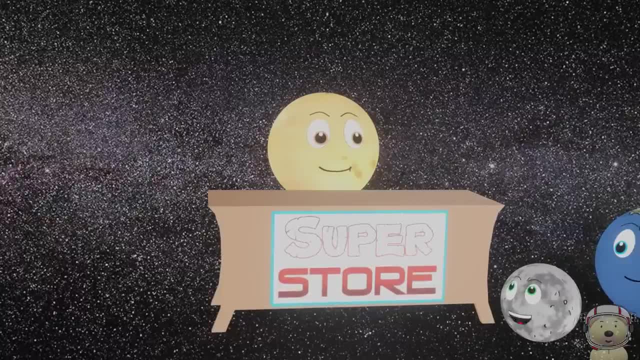 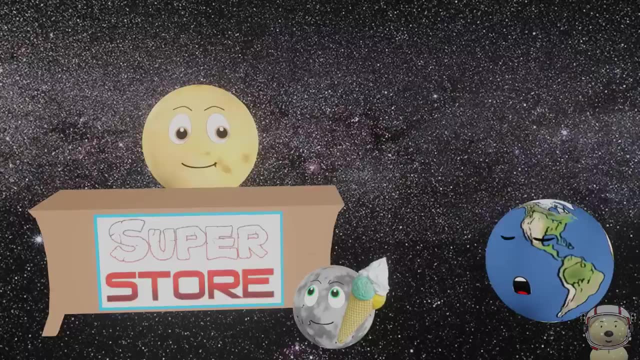 Phew Closest to the sun. Hot Ice cream please? Oh, come on. She won't have ice cream out here. Here you go, Merc Enjoy. Here you go, Merc Enjoy. Thank you, Venus. 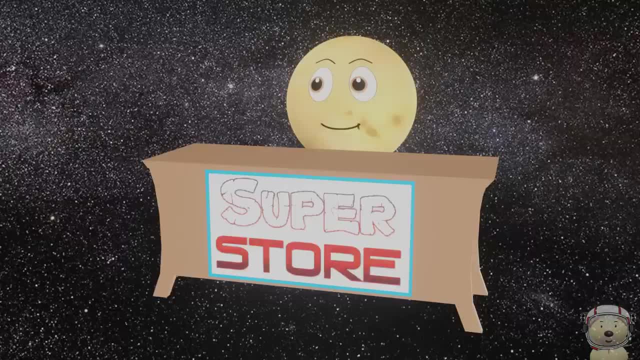 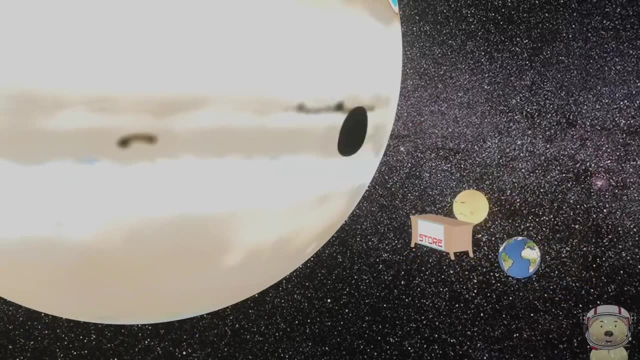 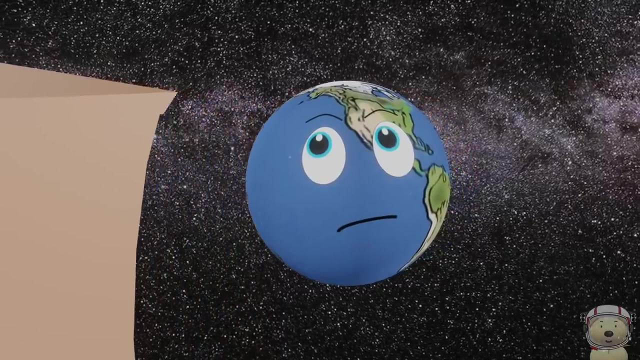 Thank you, Venus. Thank you, Venus. Who is next? Hey, Venus, I'm called the king of planets, But I need a crown. Do you have any? Yes, of course. What? Here you go. Uh, That won't fit me. 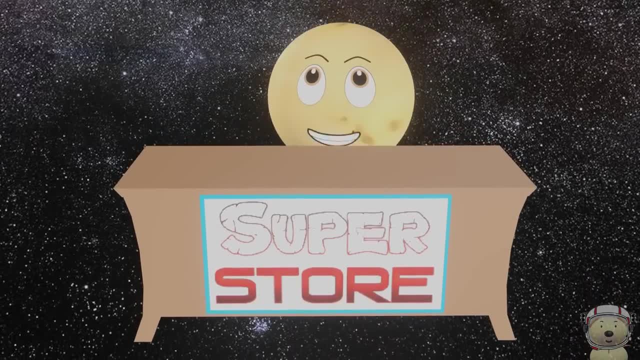 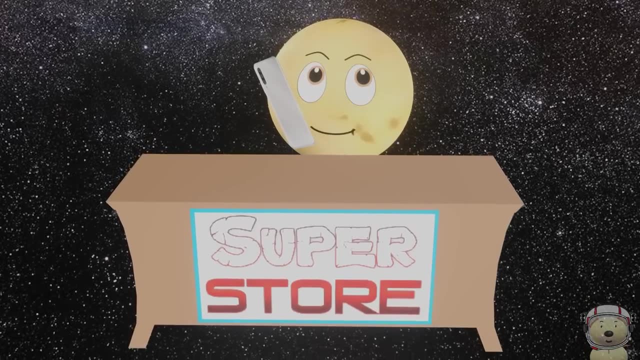 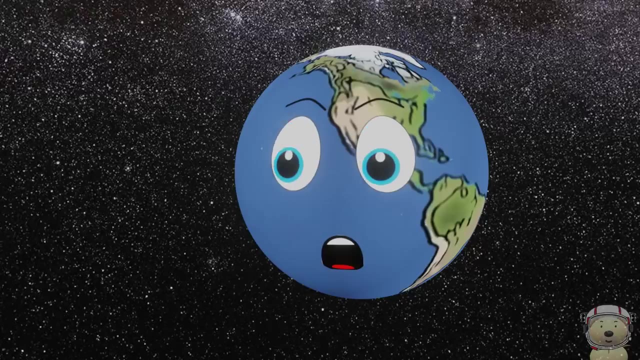 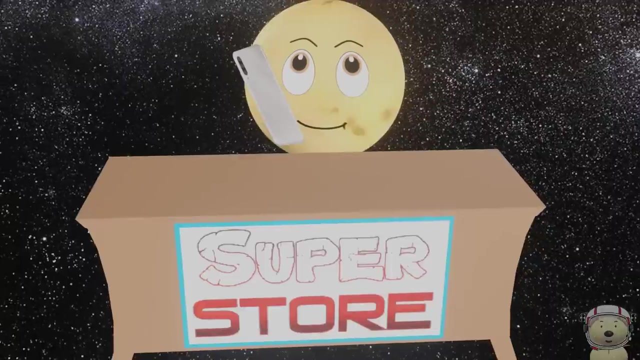 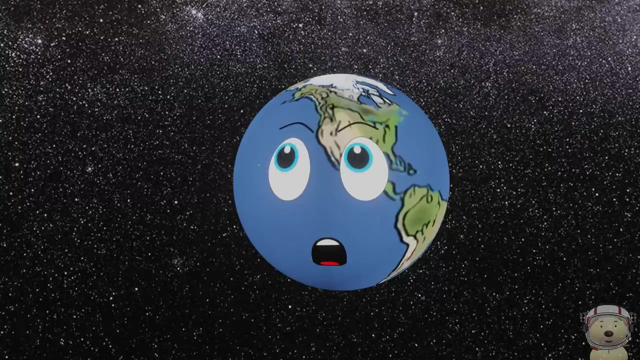 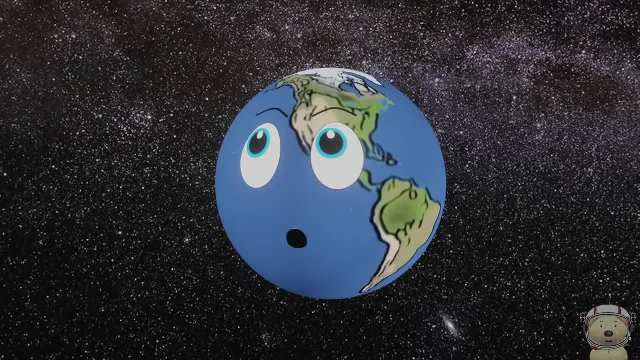 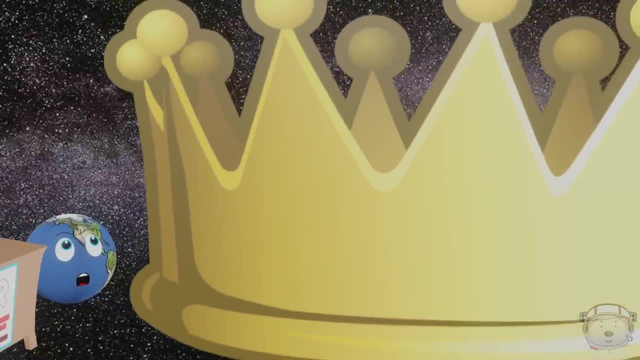 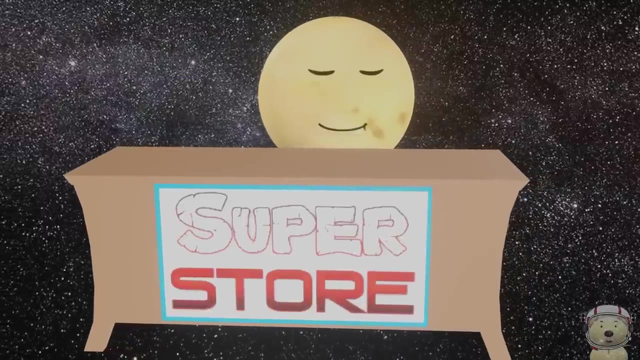 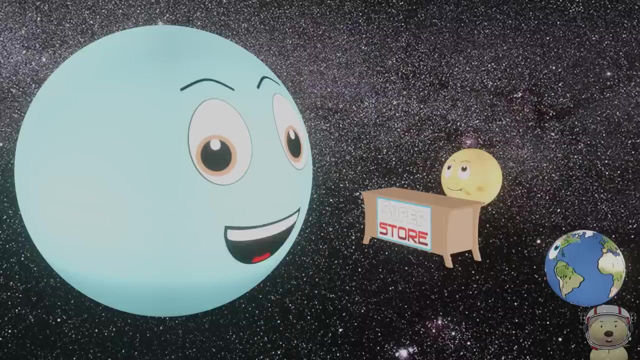 extra large please. It will take too long to cut. Ah, here it is King coming through. Hey Uranus, what can I get you? A smile, Stop that. Well, I have 27 moons, so it gets very loud. 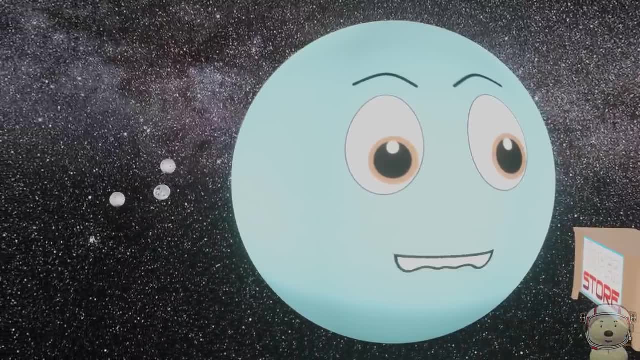 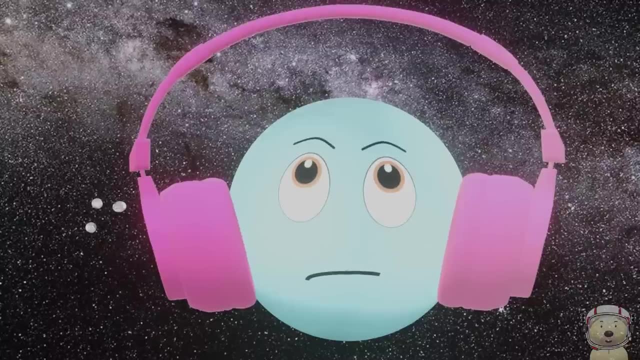 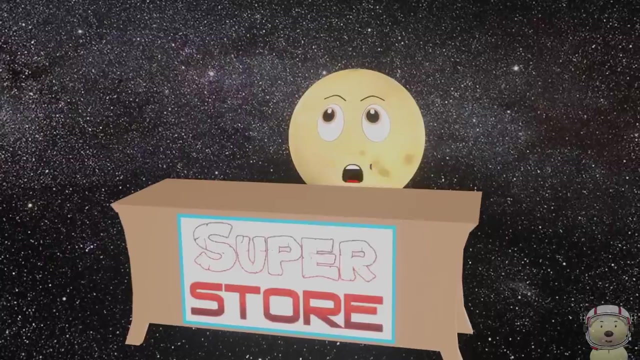 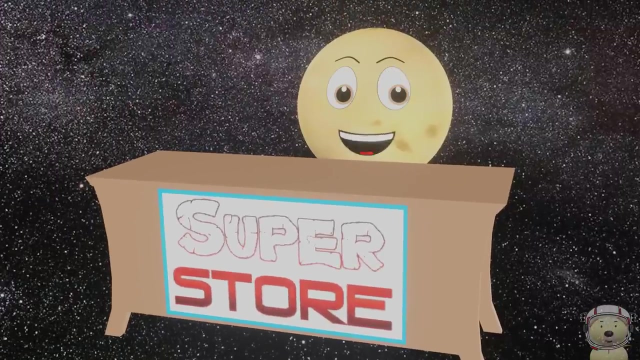 I would like a lovely pair of earmuffs to drown out the sound. Here you go. Ooh, I even like the colour. Goodness me, you're happy That's a first Venus. It's fine. You can't hear me with the earmuffs on.